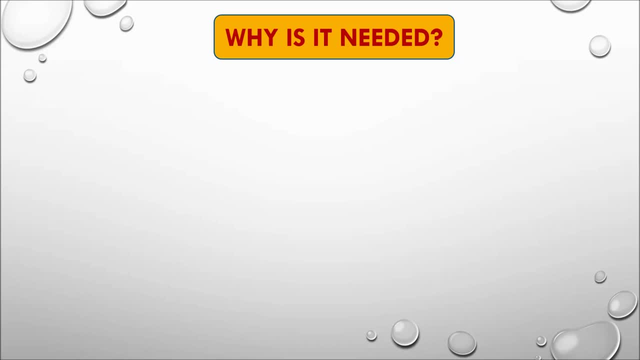 So why is it needed? That must be addressed. It is needed because it is mandatory for the fundamental geographical research to collect primary data. Alright, so it becomes a mandatory tool because we need a database and for database, data collection is the fundamental part. 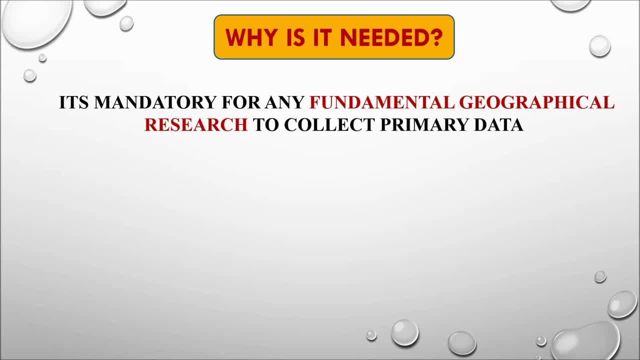 So it's mandatory for any fundamental geographical research or social science research to collect primary data And Because, especially cases where secondary data is not available or it is insufficient, it means if those data that we already have through various sources, which are secondary in nature, if they are not sufficient, if they do not cater to our 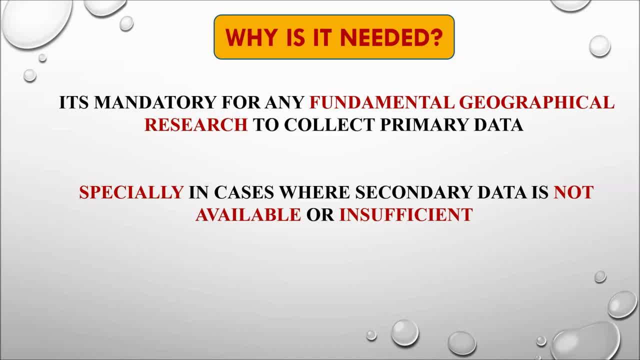 research questions as a whole. if they do not give us answers of what we are looking forward to, then in those cases it is mandatory that we have fieldwork. so fieldwork becomes one of the most important aspects where data is not available or insufficient or maybe not reliable. so in these cases, fieldwork. 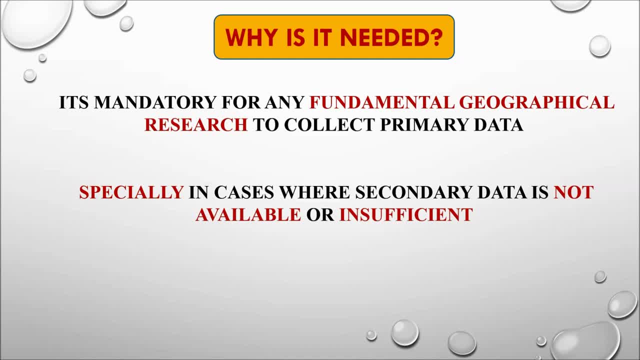 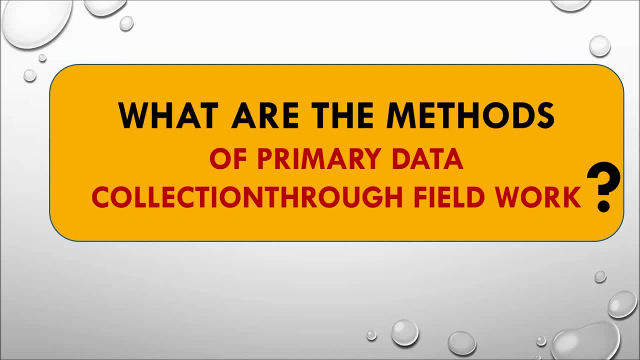 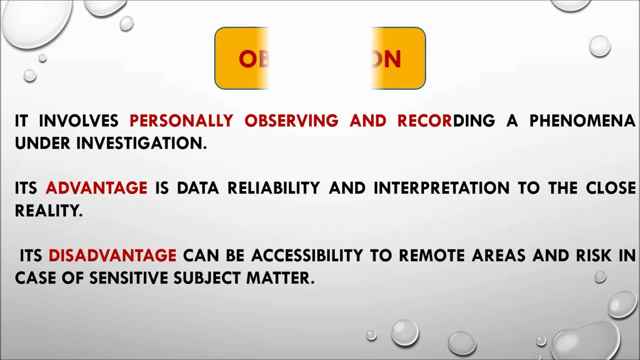 becomes the most important mandatory work all right now. so the question arises: what are the methods of primary data collection through the fieldwork? so let's look at the methods now. so first method is observation, and it involves personalization. you personally observe and record phenomena under investigation. so 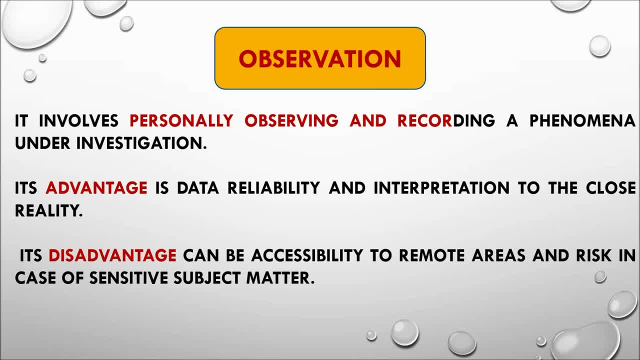 you are doing it as a field researcher. you're yourself observing and recording phenomena or an event that is happening. so what is its advantage? first advantage is that it is reliable. it is the first hand information and you yourself are aware of what you actually need. right and interpretation is 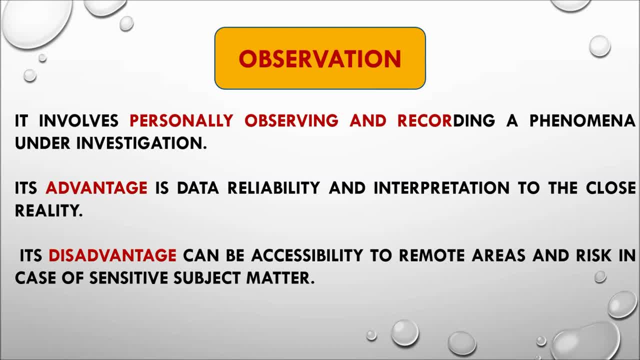 actually dependent upon how you perceive the field yourself, how you observe it yourself. so interpretation becomes really close to reality in observation and the disadvantage can be that accessibility to remote areas and risk in certain sensitive subject matters. so if it is a risky subject matter where there is a problem involved, for example if you are going to an area where 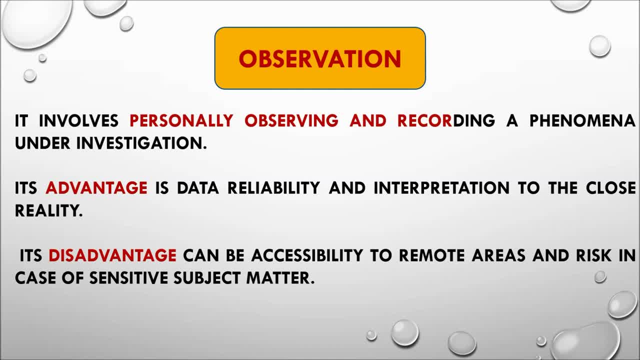 there is a hostile situation, post riots, or maybe there is a famine going on, or if there is some kind of calamity, natural calamity, or it is a remote area where accessibility is a difficult part, then you have a disadvantage of observation because you cannot directly observe it very 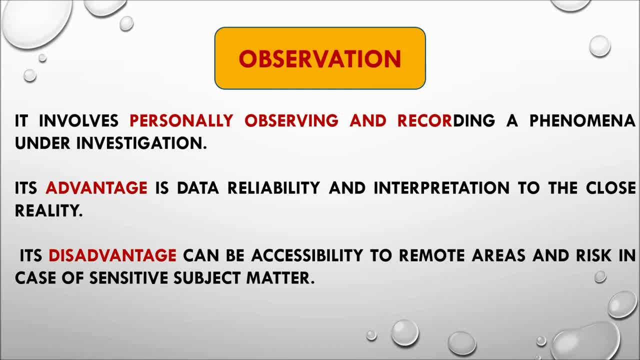 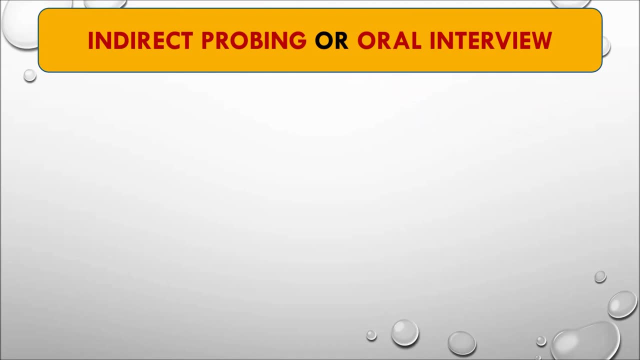 going to the field is not a feasible option, so this is one disadvantage, but the major advantage is the reliability part. okay now the second is indirect probing or oral interview. this becomes really important in data collection because it considers of the collection of data by the researcher in an indirect manner. okay, so 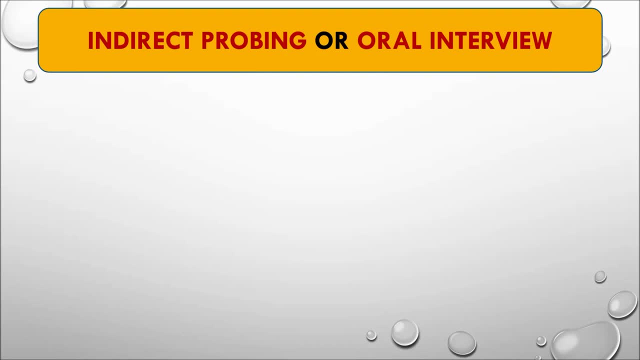 what is that manner? let's see. so this method of data collection ensures first-hand information. okay, because the interviewers can cross question for the right and appropriate information. okay, so there is cross questioning involved while we are talking, where we are probing. all right, so this is very much. 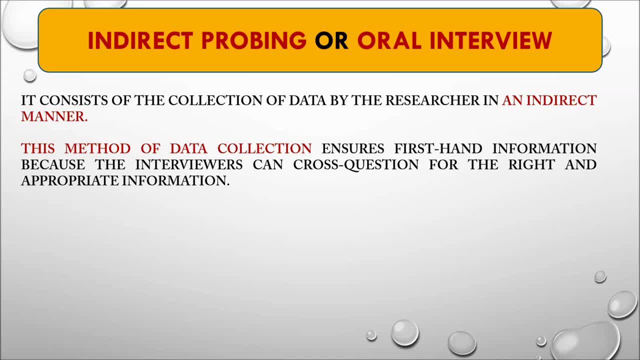 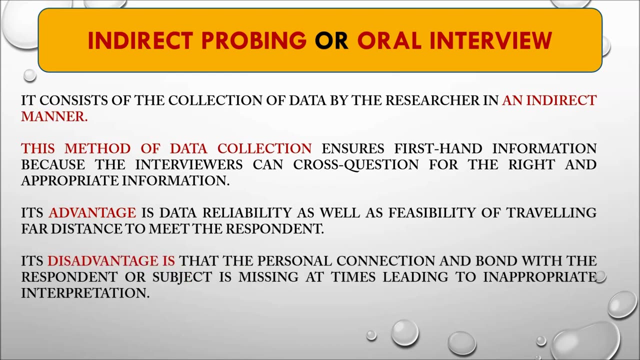 important that it ensures the quality of the data by cross questions- okay. and advantages that data is reliable as well as feasible, because it restricts the traveling part to far distances- okay, so we can call a person and talk about it, we can probe a person, we can do that orally, all right. and disadvantage is 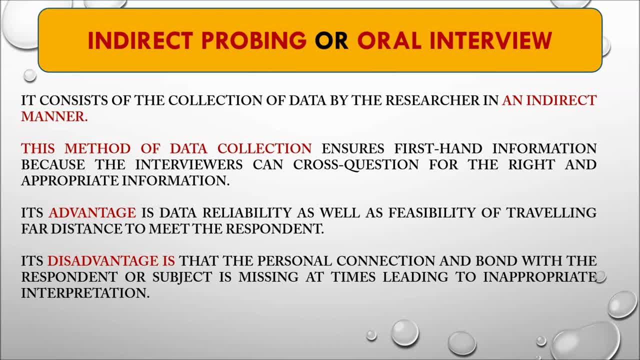 that the person need a connection, a bond with the respondent or subject is missing at times, leading to inappropriate interpretation. so what is the disadvantage in this case? you don't have a personal connection that you build when you go to the interviewer and you don't have a personal connection. 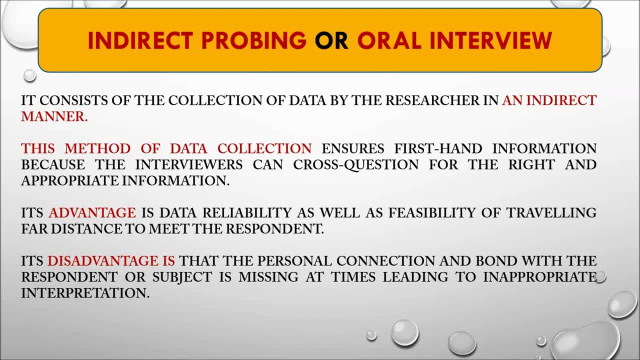 okay, so many times this, this linkage, is not there exactly what we say. so what happens? many time it leads to inappropriate interpretation of what a person is saying through the interview. so that is one disadvantage of this method. now the next method is direct personal investigation. so when you are 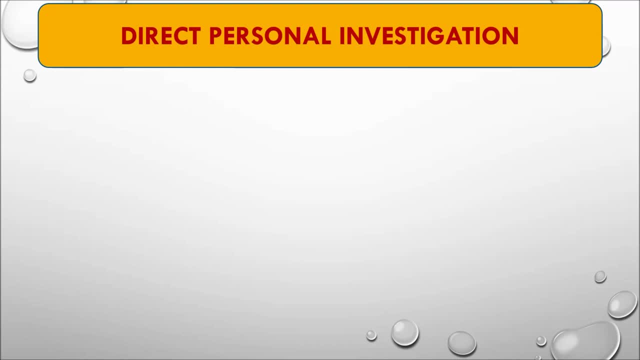 doing it direct, personally, it becomes very much important. so it consists of the collection of data by investigator or the researcher and the person who is the researcher in a direct manner. so a researcher himself enters the field and asks, solicits the data that he requires. okay, so this method of collection, 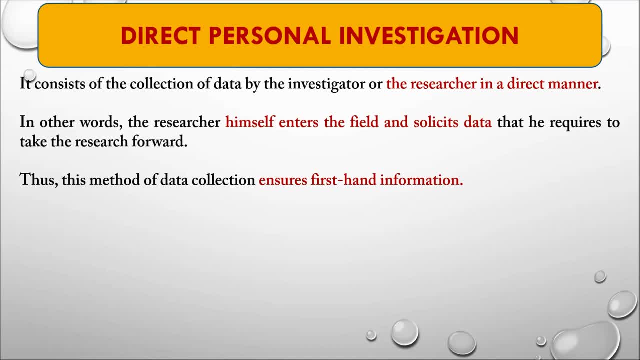 ensures firsthand information. that is important and it is reliable for an intensive research. so if you are having an intensive research that you are doing in your research, you must understand what is an intensive or an extensive research. an extensive research will have lots of objectives and a huge amount of 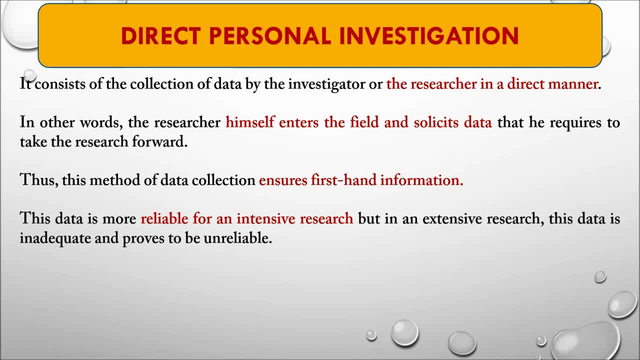 huge area to cover but an intensive research. it's a small area, a small objective, limited objective, but more of the investigation that is personally based, all right. so this data is inadequate at times for extensive researches that we say so. it is also time-consuming that we need to. 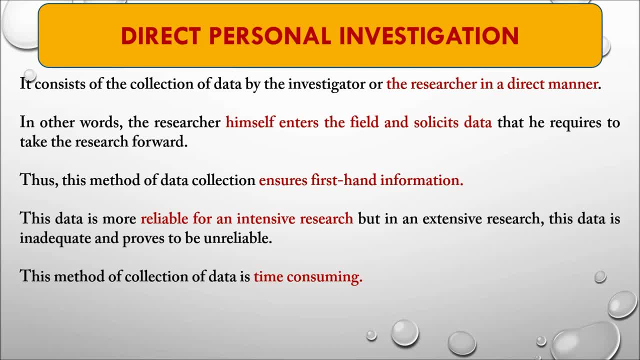 understand. and the greatest demerit of this method is it is very subjective in nature. why? because it's not suitable for objective based, extensive researches. okay, so it can be subjective. it can be prone to different interpretations because the researcher may have a different thought process, a different point of view. if you say so, this can be questioned at many. 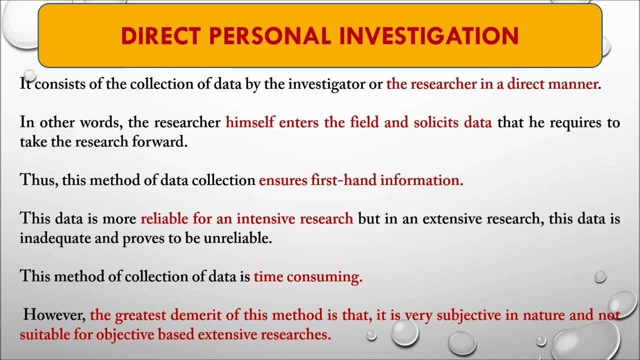 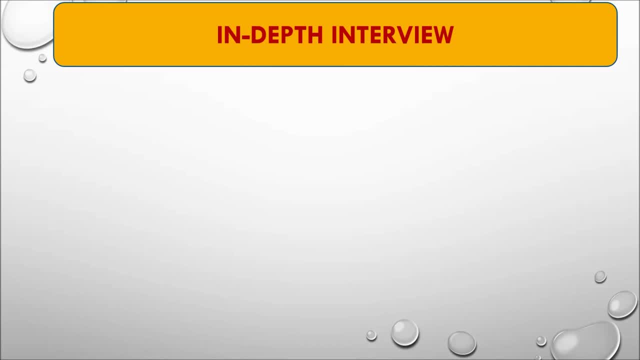 platforms while we are reporting it or publishing it all right now. the next is in-depth interview, very famous because of the biographies coming into the picture in the research market. so what happens? it is a qualitative research method, first of all. it is a qualitative research method. first of all, it is a 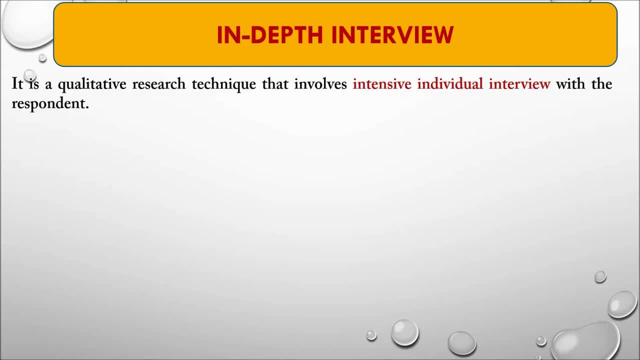 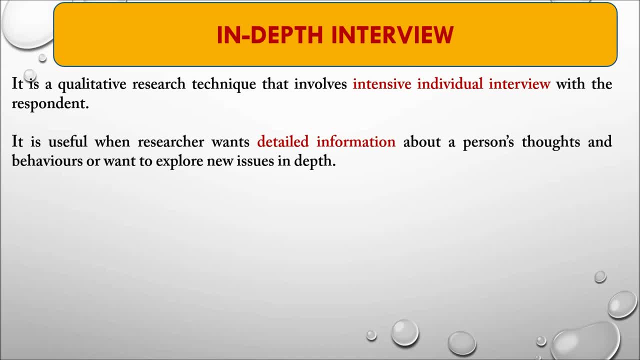 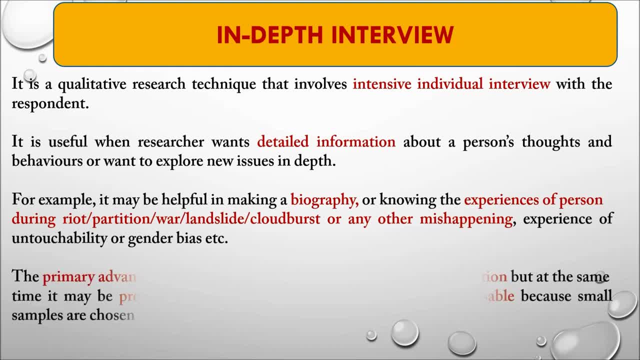 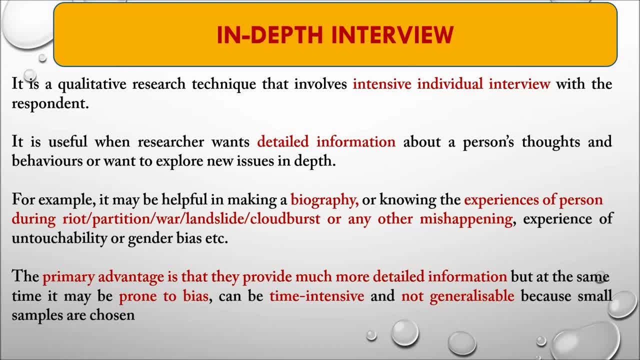 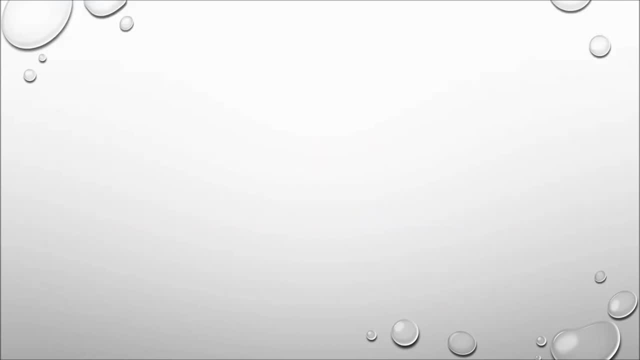 of biographical interviews and also it's not generalizable because it's very individualistic, isn't it? so general theories cannot be woven around these samples, all right. so that is the disadvantage of in-depth interview. now, then, we have mailed questionnaire survey, as it is there that we have to mail the questionnaire to the respondent and respondent will fill it up and 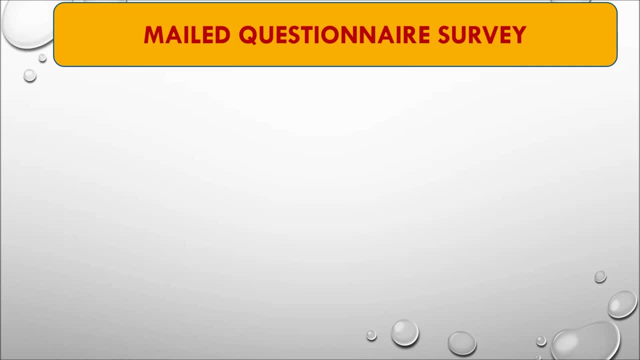 send it back to us. so what happens? it consists of mailing a set of series of questions related to the research, for which respondent would answer, and then it will come back to the researcher. so this method of collection of data is time-saving, cost-efficient. these are the advantages that we 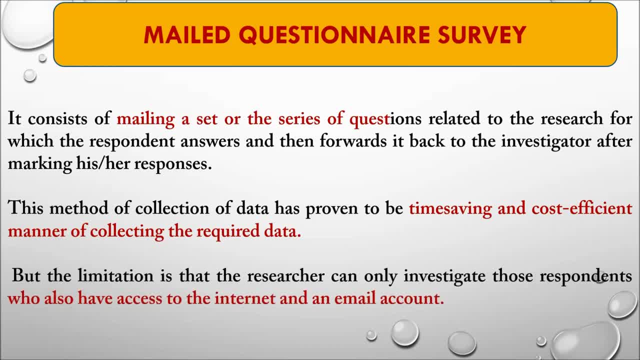 say, but limitation is that researcher can only investigate those respondents, in this case, who have access to email and internet, isn't it? and also it's important that the person is aware about the respondents and has a personal bond. in that case, a person need not travel. it's not necessary that a person has to travel in that case. all right then. next is the. 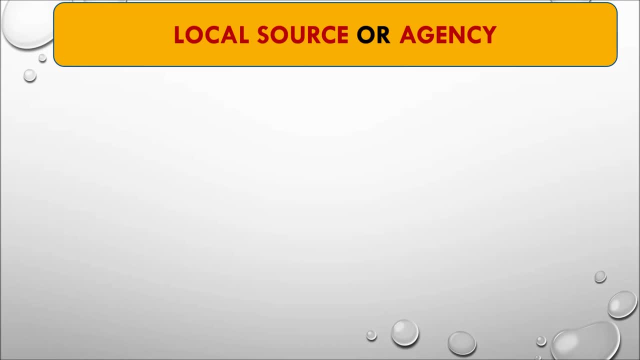 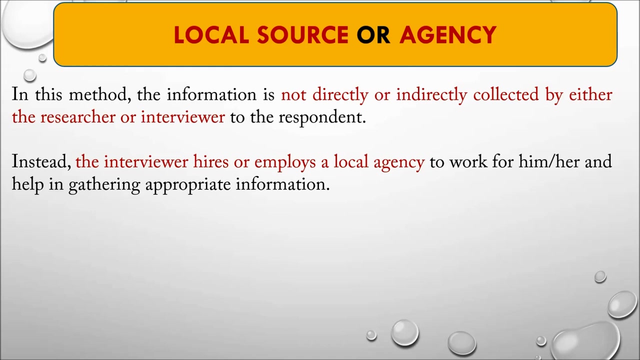 local source or agency method. so what happens in this case? the researcher directly or indirectly collect their data through this method. okay, which is local source based or agency based? in this case, the interview hires or employs a local agency to work for him. so if I am a researcher, I'll pay that. 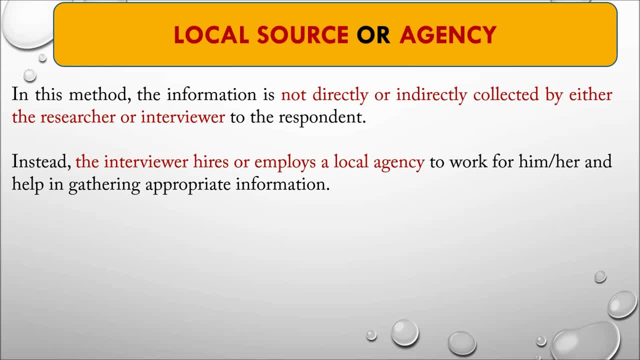 agency that you please collect this data on behalf of me. so this cases are known as correspondent people, correspondent database. so what happens? these people who are local agents, are known as correspondence, who are responsible for gathering or collecting the accurate or reliable information from the field. but it may be costly and also, again, because it's not directly involvement of the 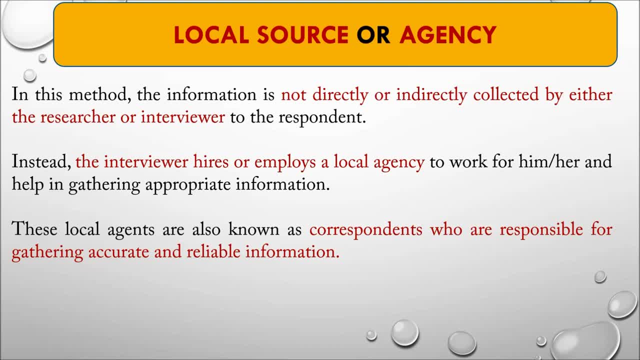 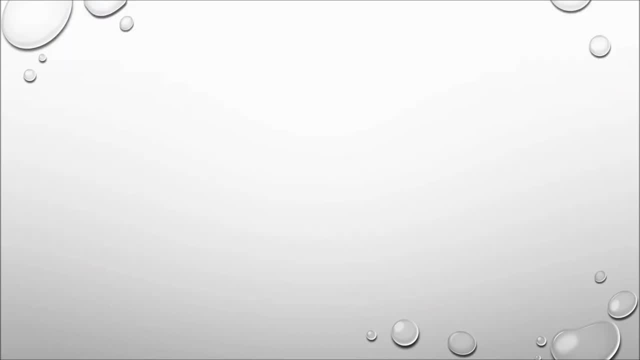 researcher. reliability and interpretation may be a question in this case. again and then again, what we have learned is the in-depth interview, that that is important in this case and further, what is there is the schedules and the questionnaire. so schedules and the questionnaire are sometimes interchangeably used. okay, so remember, schedules and questionnaires are. 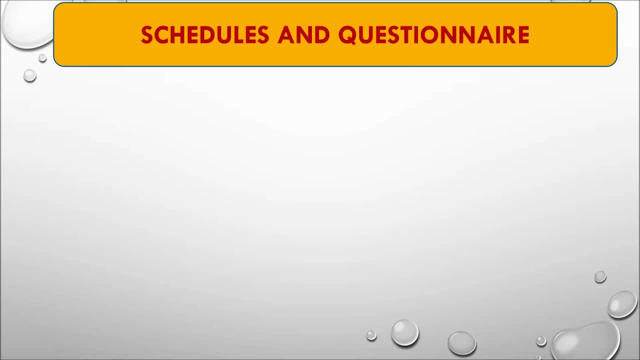 interchangeably used, but it is different. schedule is different and questionnaire is different. how, let's see? so it involves a face-to-face situation with the respondents. so we go to the respondents, sit with them and talk and do this scheduling and interview. so what is that? the interview questions. 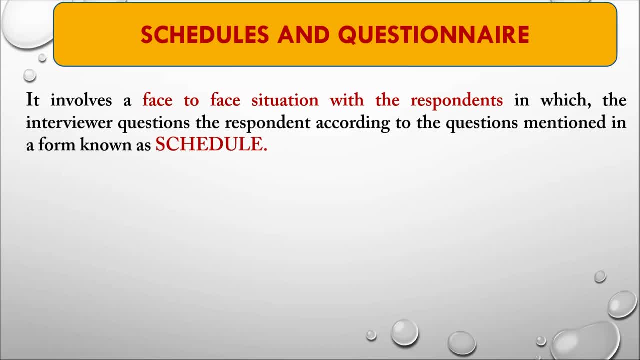 the respondent according to the questions mentioned in the form that is scheduled. so what happens? a researcher designs a schedule which has lots of questions related to the research that you want to obtain data for. okay, so this kind of method is called scheduling. okay, this is different from a. 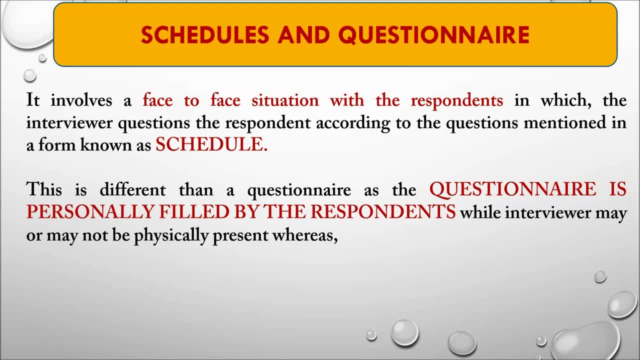 questionnaire, as questionnaire is personally filled by the respondents, while interviewer may or may not be physically present. so it means questionnaire is not filled by the researcher, okay, it's filled by the respondent, okay. but if it is schedule, it means that our researcher is sitting with the respondent and 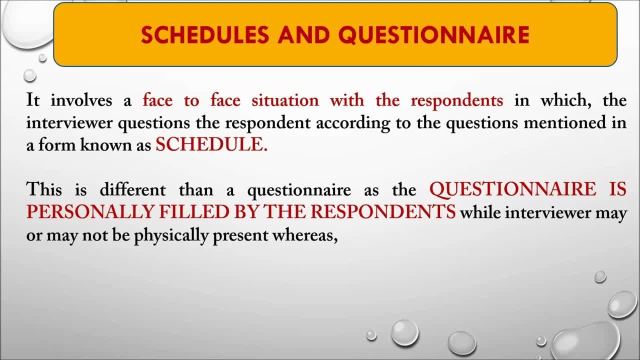 filling it just by asking questions. all right, so the schedule is filled by the researcher and questionnaire is filled by the respondent. that is the basic difference. so always remember, do not confuse between schedules and questionnaire. whenever you are preparing for a field work, we always say: make the questionnaire. but are we making a questionnaire? is it really a questionnaire? 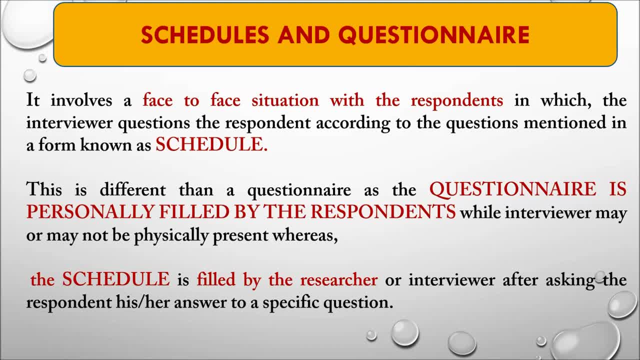 unless we are making it in the language of the respondents. it's not a questionnaire, because we are making schedules. we are putting lots of questions and we are asking them and then we are filling it. the respondent is not filling it, so in that case it's schedule. so remember, if you are 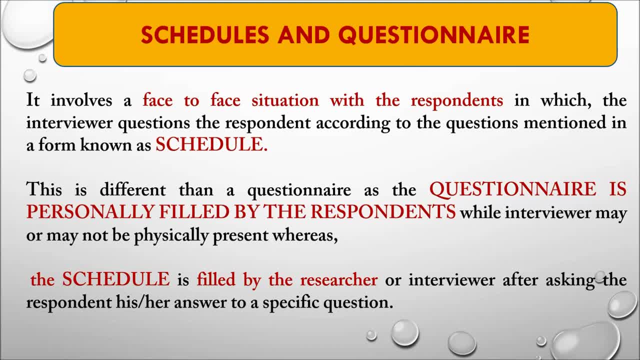 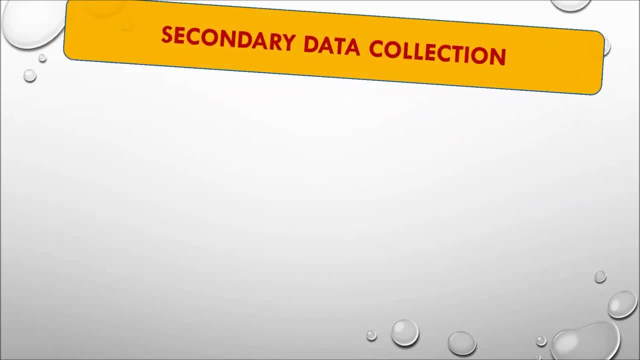 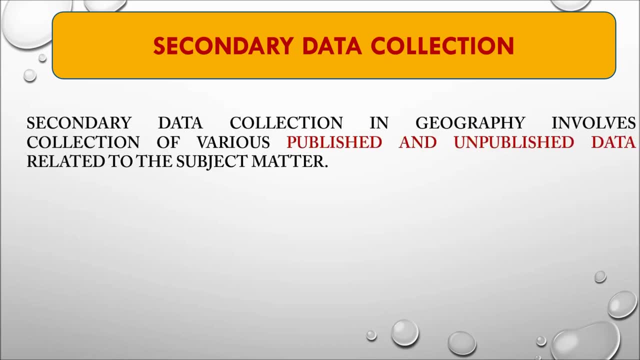 scheduling it or making a questionnaire so clear your myths in this case, all right. and then, after all these methods of primary data collection, a little inside of the secondary data collection. so what happens in secondary data collection? it involves the collection of various published and obviously unpublished data as well, for various 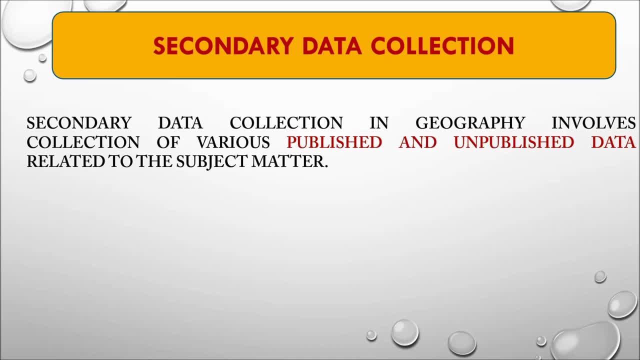 related subject matters, so it needs a careful investigation because it's not direct, isn't it? it has to be based on somebody else, so reliability is under question and results have to always be verified by conducting field work. so ground truthing exercises during field work is also. 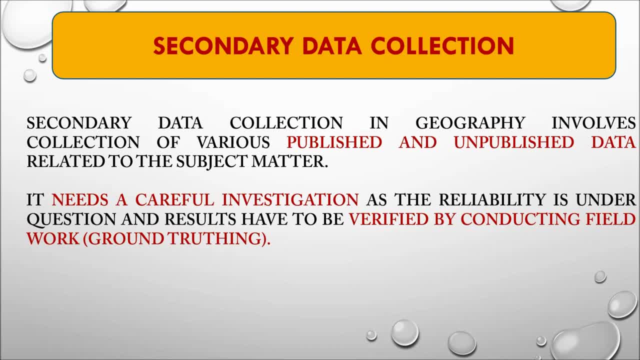 based on secondary data. so if suppose I get a data about a particular area from some source, we must verify it before arriving to any interpretation, any conclusion. so the sources that majorly we seek is government websites and offices- isn't it- and publications, reports and other compilations. so 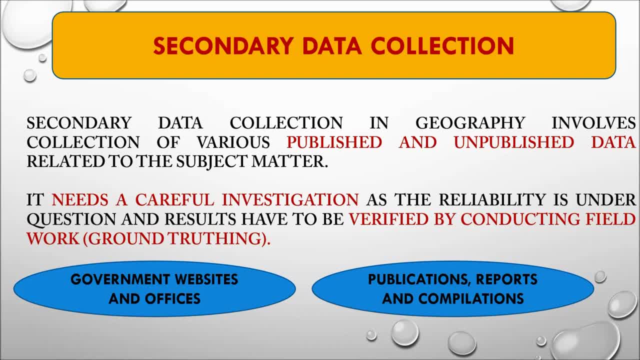 these are the major secondary data sources, but remember to always relate the secondary data to the ground. that is how its reliability can be verified. so this is all about the methods of data collection in the field work in today's session 7, so please like and subscribe to our channel: the geocologist.